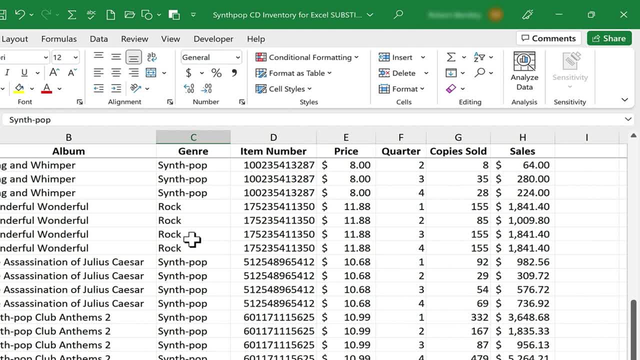 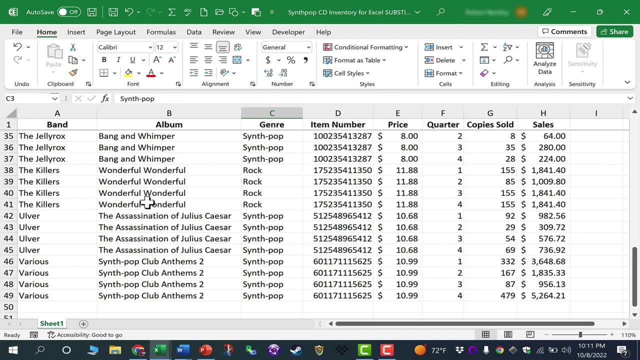 find and replace isn't really what you want. You may want to just change the text in a specific range or in a specific cell. So, for example, here at the left I have a list of synth pop albums and other related genres And you can see. 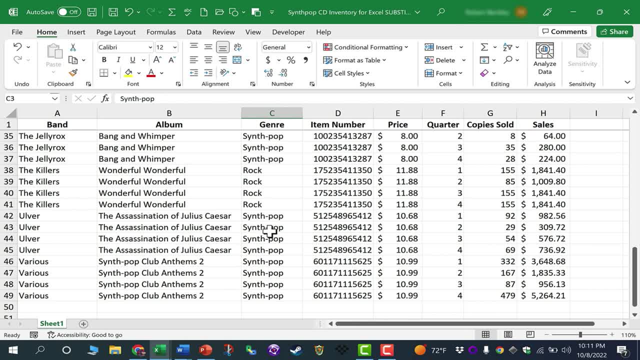 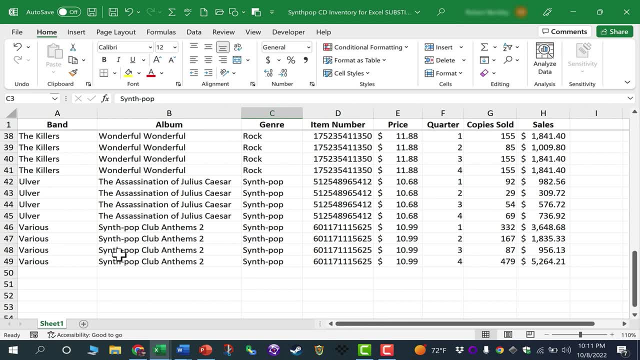 here that find and replace changed not only the list of genres but also the names of some of the albums. This album was named not by me but by someone else, And the official name of this album does not have a hyphen in it, So that's not really accurate for me to go ahead and just change the title of 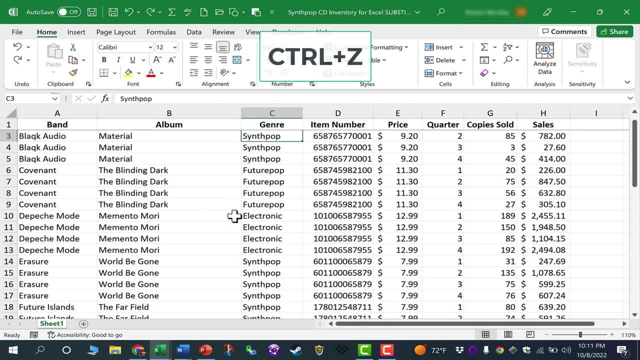 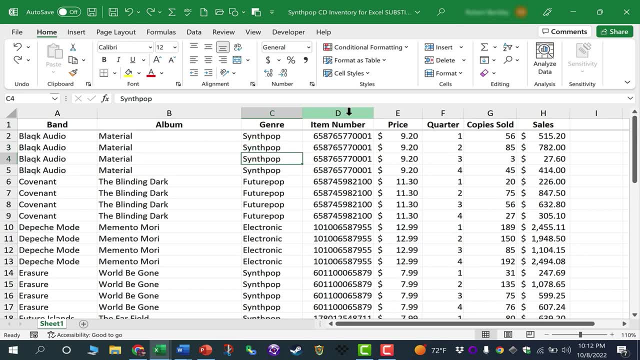 this album that someone else produced, So I'm gonna undo that with ctrl Z on the keyboard. Instead of using find and replace, I'm gonna use the substitute function. Step one in this case is: I need some space to work with, So I'm going to. 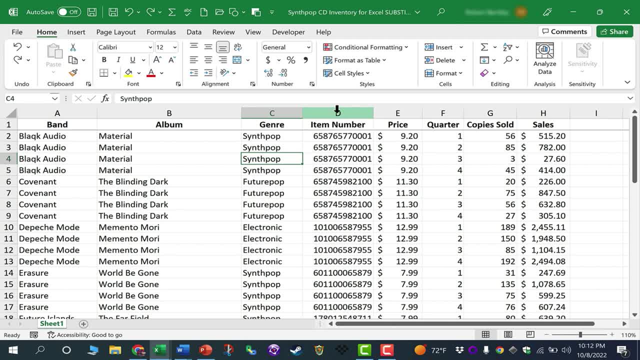 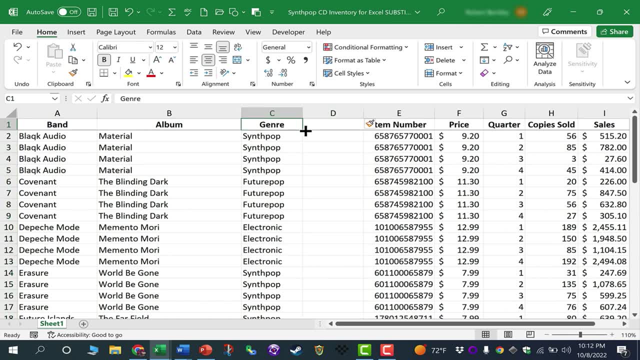 insert a new column between C and D. I'll do that by right-clicking on column D and now I have that blank column And I'll click here on C1 and use the autofill handle to just drag that over. so that genre is repeated here in column D Next. 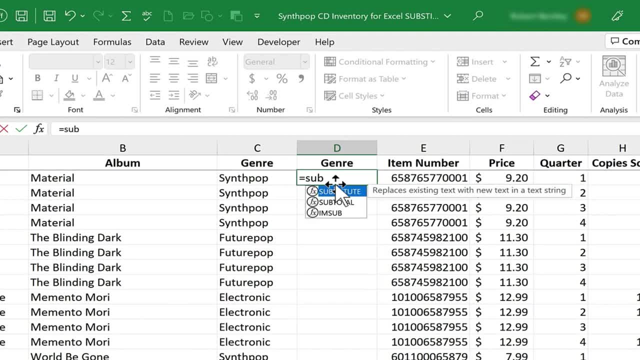 I click on D2 and I'll type equals- substitute. As soon as I start typing that, you can see Excel is suggesting the substitute function. It says it replaces existing text with new text in a text string. That's exactly what I want to do. 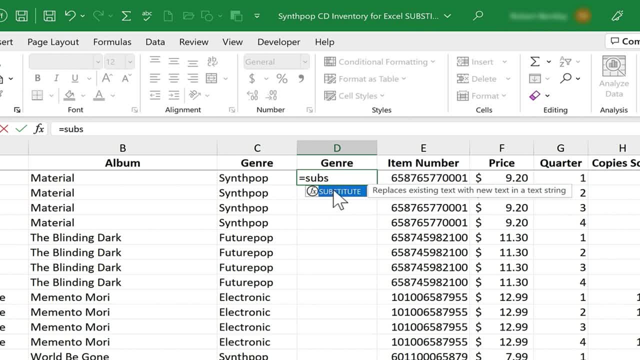 So I could just continue typing the word substitute. It's kind of a long word, though, in this case, but it's not enough, So it's fine. Now I'm going to go ahead and case, And I think I'll just double click here on substitute, and it puts in that function for me. 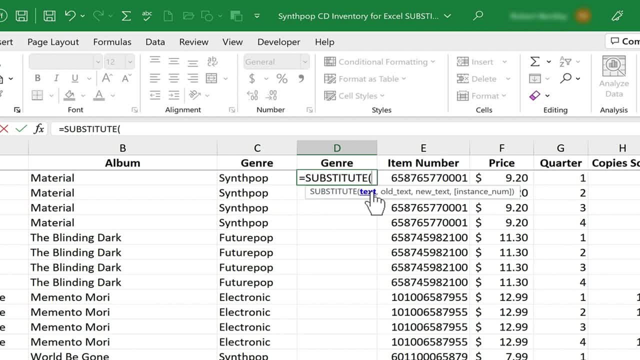 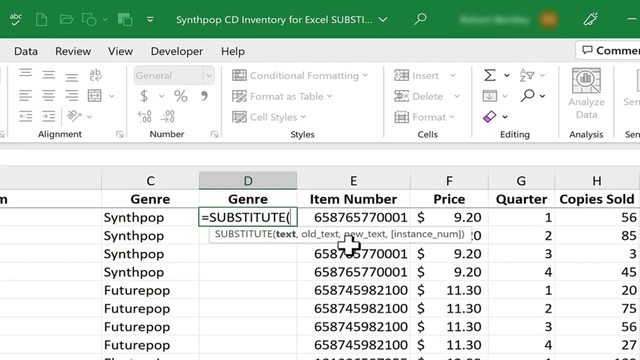 along with a left parenthesis. And now Excel gives me a little pop-up that gives me hints about what Excel is expecting me to provide to it. It's expecting me to select some text, put a comma and then type in the old text, the existing text, comma and then new text, And then there's another. 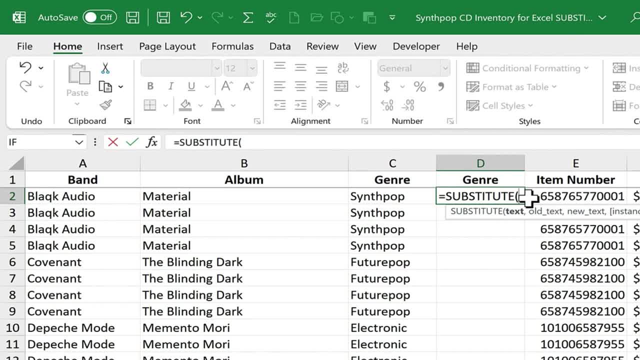 optional thing here at the right. Let's talk about that later, But for now I'm just going to click on C2, or I could type the cell reference C2.. But either way, I'm showing Excel that this is where the text is. I'll type a comma. What is the old text In quotation marks? I'm going to type: 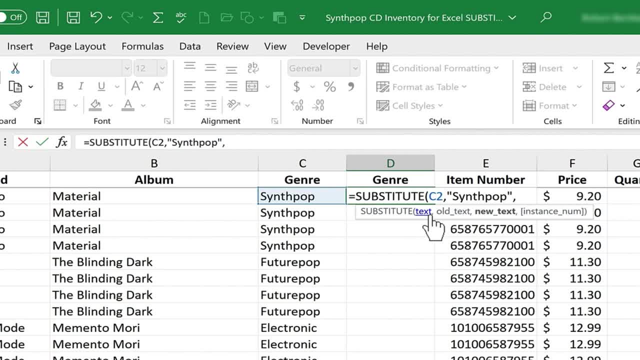 synthpop. close quote: I put in my comma. Now, what's the new text? What do I want to change this word into? Again, it needs to be in quotation marks. I'll type in synth, hyphen and then comma, And then I'll type in the old text And then I'll type in the new text. 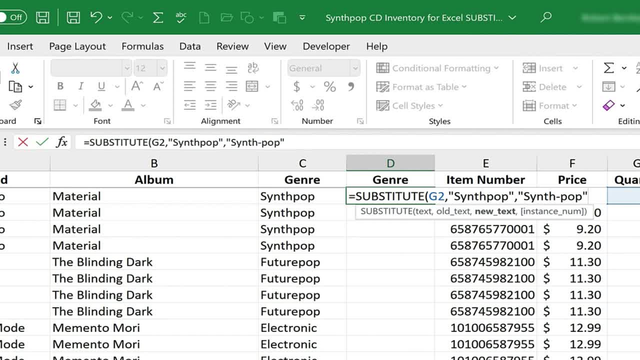 Synthpop. close quote: And that's all that's required in this formula. I should put in my right parenthesis, but in this case I don't really have to, And then I'll just tap enter on the keyboard, and it didn't work Somehow when I was typing out the formula, the cell reference. 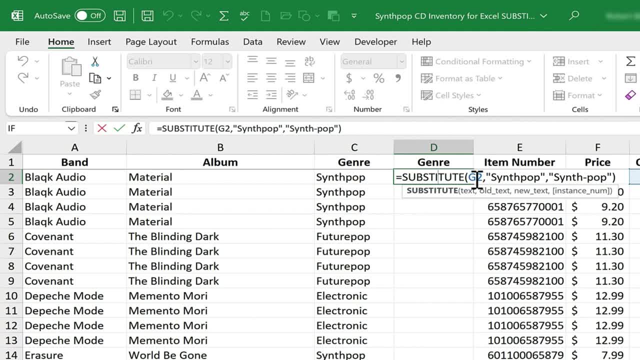 C2 became G2.. So I'm not exactly sure what I did wrong there, but I'm just going to change that from G2 to C2, tap enter, and it worked. Now do I need to do that same formula over and over? 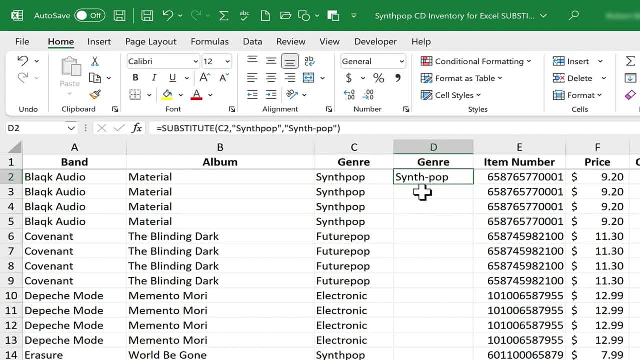 all the way down this spreadsheet. No, Fortunately no. I can just click here on D2, where it looks like it says synthpop with a hyphen. But actually what's in this cell is this formula here that you can see on the. 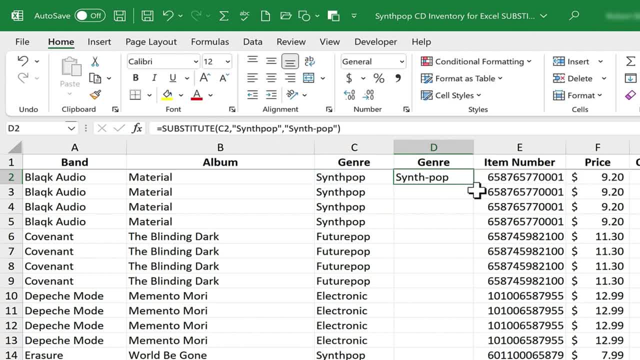 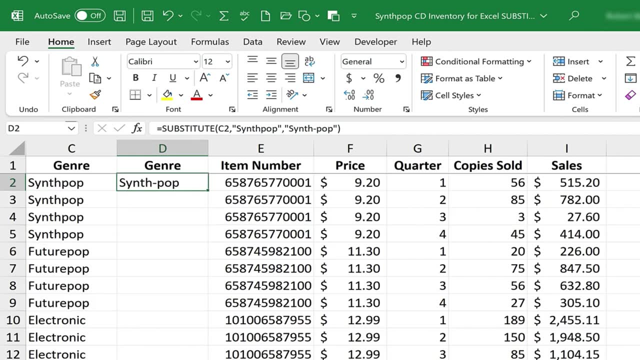 formula bar. So with that cell selected I can just double click in the lower right-hand corner of the selected cell. There's an autofill handle there. In this case it's so small it's hard to see, but there it is. It's just this small green square. I'm going to go back to a more zoomed. 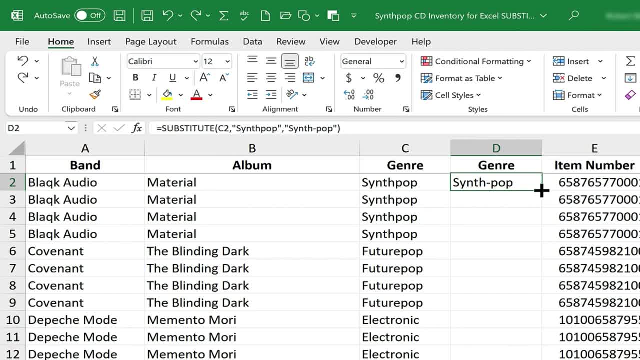 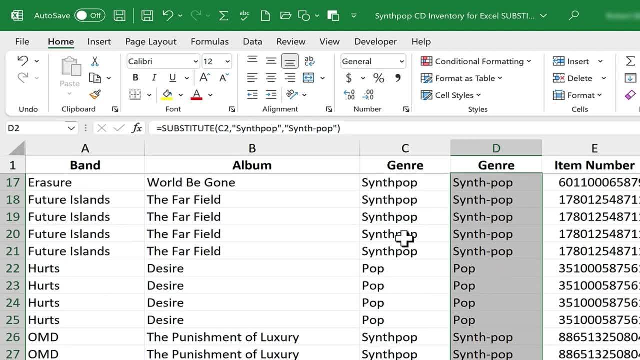 out view. I'm just going to double click on that autofill handle and look what happens. It copies that formula down the spreadsheet and it's looking for synthpop without the hyphen and changing it into synthpop with a hyphen. Now what if it doesn't find the word synthpop? That's okay, It. 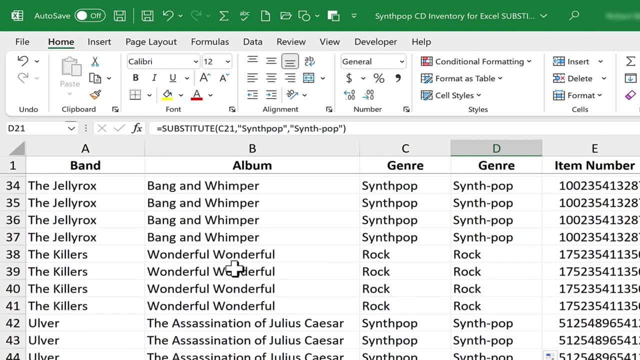 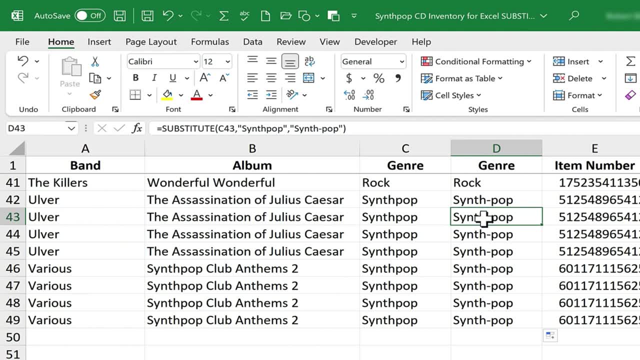 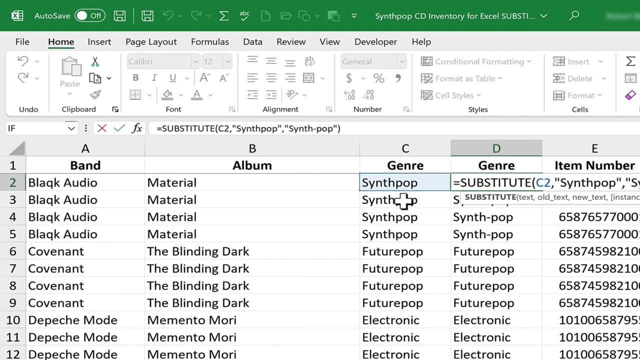 just keeps what was there already. Now, what about my album that's called Synthpop Club Albums 2? That was not changed. Why? Because I used the substitute function. Excel is looking specifically at the column and the cell, in this case, that I put into the formula, So C2.. That's where it's. 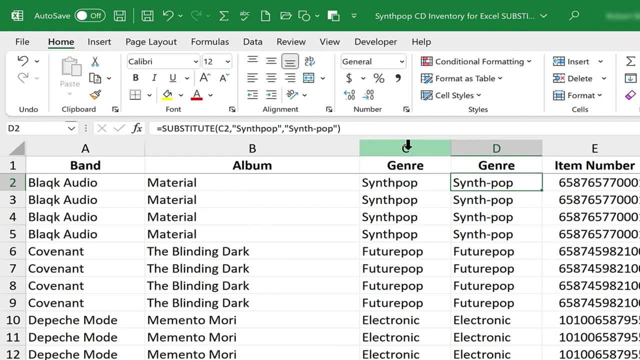 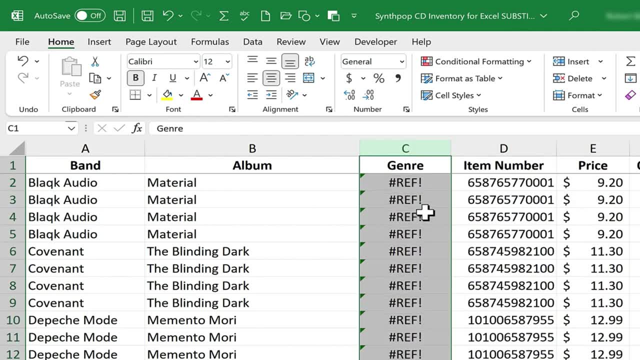 looking, It doesn't care about column B. Now at this point I'm tempted just to delete column C. I don't need both of these columns, so I could right click on C and choose delete. But look what happens: It ruins column C. So I'm going to undo that and what I'm going to do to fix this issue. 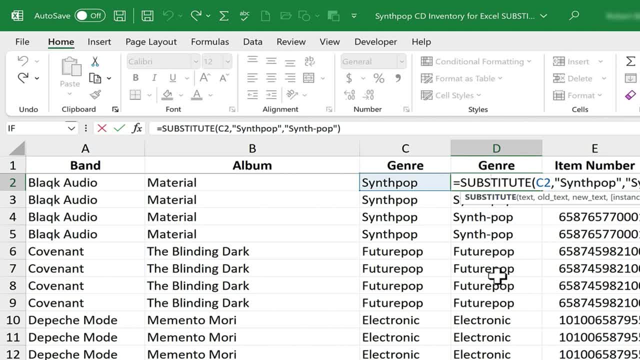 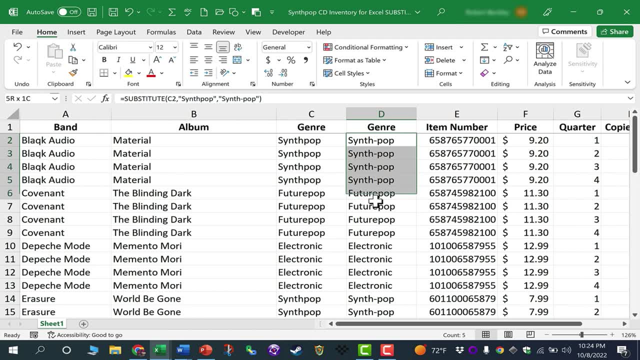 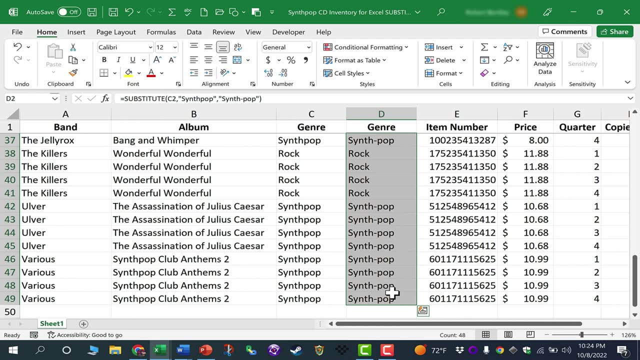 of the fact that this column now is full of not simply text but of formulas that produce text, is I'm going to click and drag to highlight the range that I would like to take from being a formula and turn it into simple text. So I've highlighted that range. Now I'll just copy it. 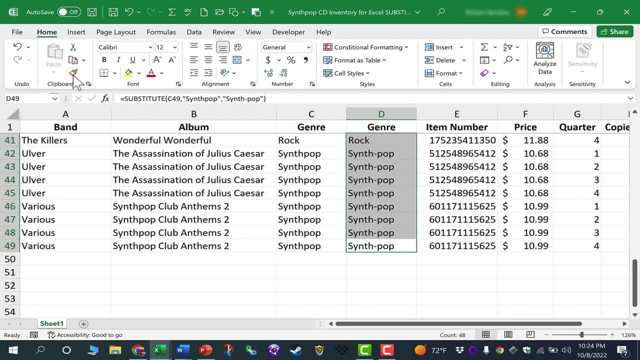 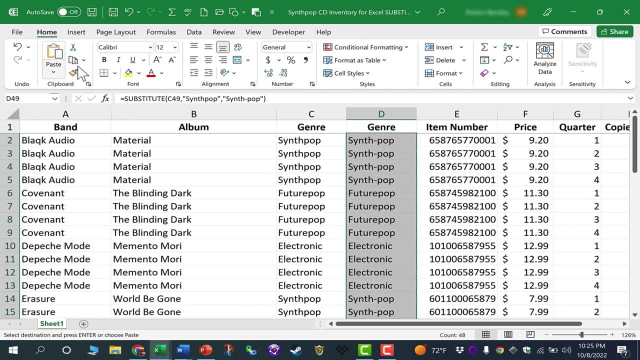 In this case I'll just go up here to the Home tab clipboard group and click on copy And then, with that same range selected, I'm going to go here again to the same clipboard group, but this time I'll click on the lower part of the paste button and I'll choose paste values. So I've 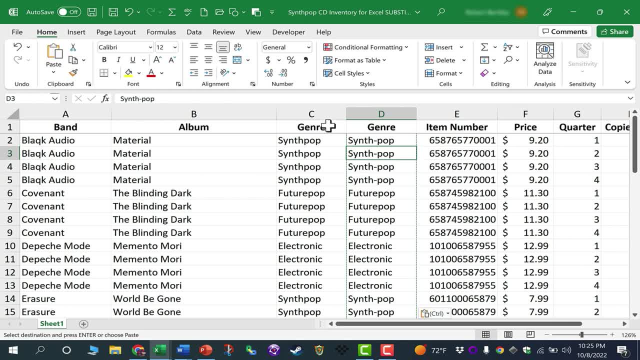 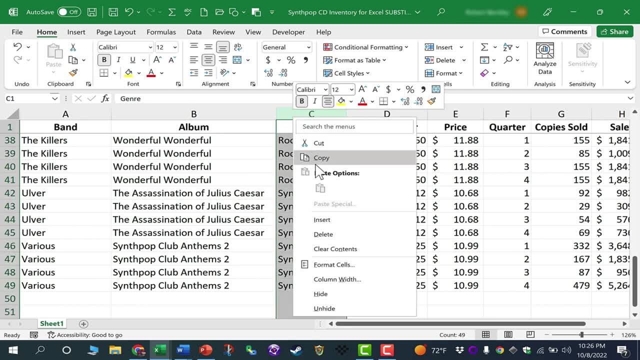 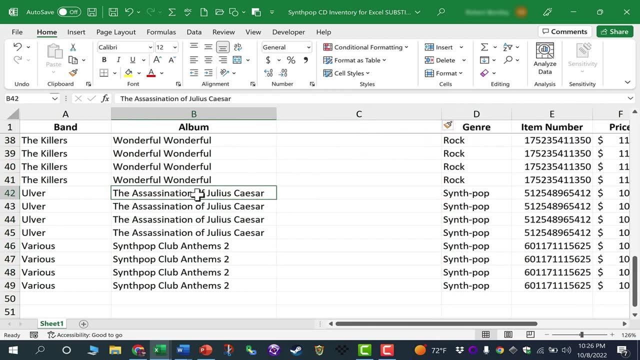 selected paste formulas and pasted values. So now I can delete column C and there are no issues, no errors. Now there's one other optional argument that you can use in your substitute formulas. So I'm going to insert a new tab to demonstrate this and I'm going to go in here to the name of this. 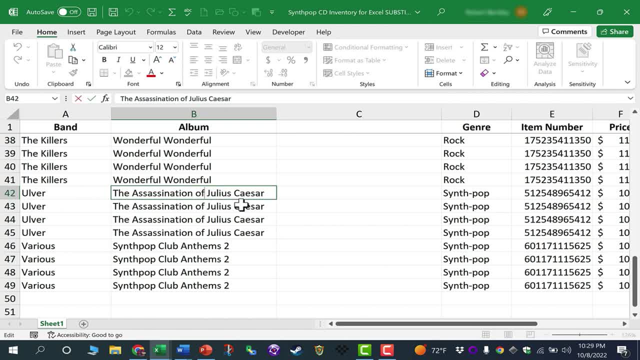 album by Ulver and I'm going to change the title of this album to make it incorrect. That's not the correct name of the album. Now let's see how could I fix that using the substitute function. I'm just going to click here on cell C42.. I'll type equals- substitute- left parenthesis. I select. 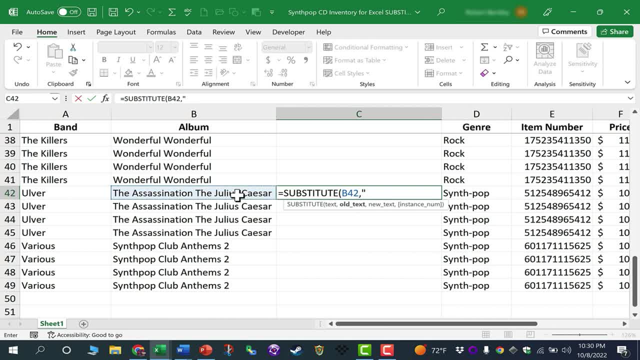 the text that I want to change. comma in quotation marks. What is the old text? It's the word the Now. keep in mind this is case sensitive, so I need to make sure that I'm typing exactly the text that I want to replace. Close quote. put in my comma the new text. in quotation marks I'll put the word of: 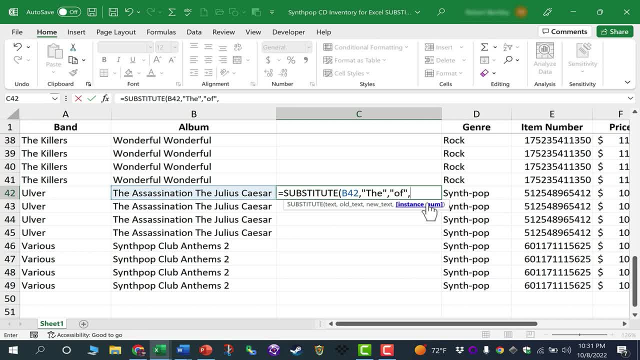 and I'm going to paste that in here. So I'm going to type the word of: And here is an optional argument that will help solve a problem. You can see the problem. Cell B42 has two instances of the word. the Which one do I want to replace with the word of? Well, in this case it's the second instance. 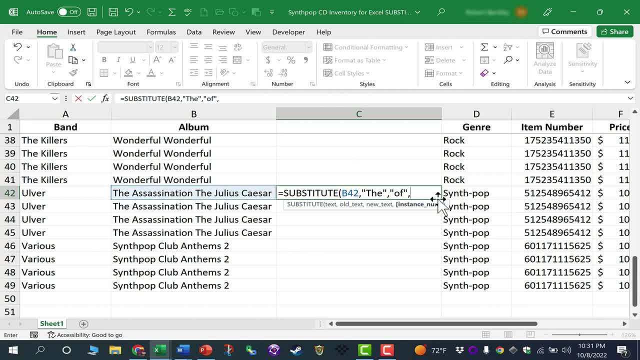 So, even though this is optional, in this case I really need to use this, because I don't want to change the first the. I want to change the second, the, So I'll just put in a number two. I should, using the substitute function. it left the first the alone, but it changed the.